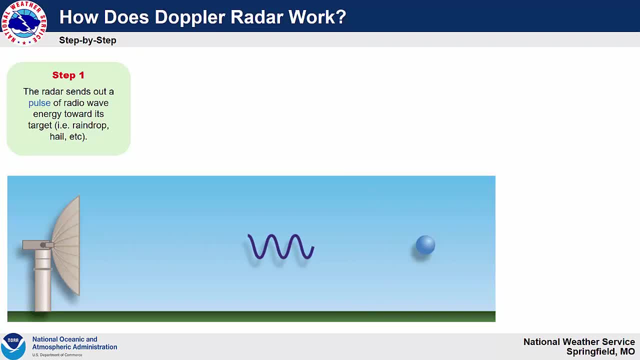 let's dive into how they actually work. Here's a step-by-step process. First, the radar sends out a quick burst of radio wave energy, called a pulse toward its target. This target can be anything really, but for weather purposes we're talking about raindrops. 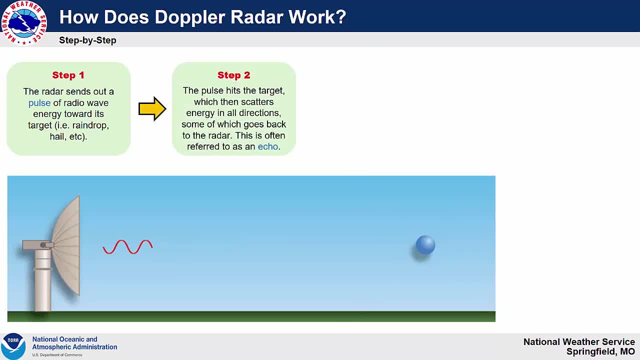 hailstones, snowflakes and so on. Once the pulse hits its target, energy is scattered in all directions, some of which goes back toward the radar. This backscattered energy is often referred to as an echo. While this is going on, the radar is simply waiting. 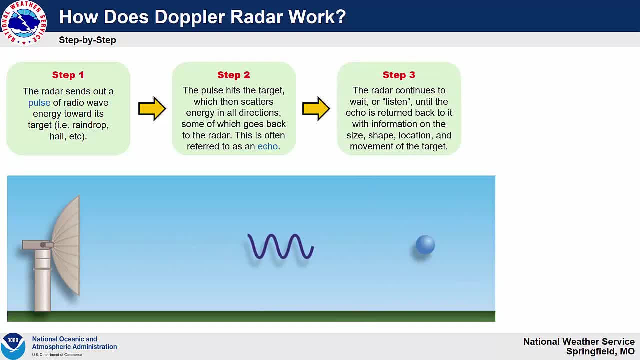 or listening until the echo is returned back to it with information on the size, shape, location and movement of the target. Finally, once the echo is received, the data are sent to a computer system that processes the signal. This information is used. 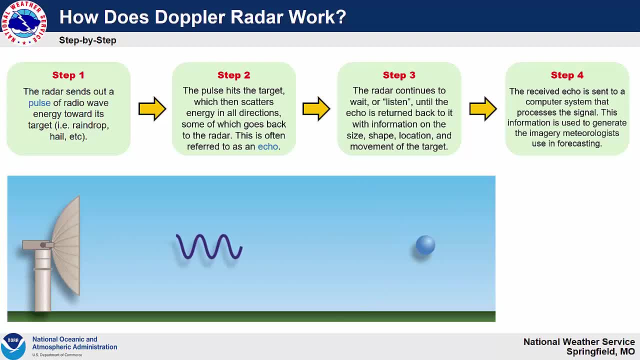 to generate the imagery meteorologists use in forecasting, like the ones you see on TV or on your smartphone app. These images look like these, and the signals that you receive from the radio are not going to look the same in any other way, because the data is sent to the computer system. 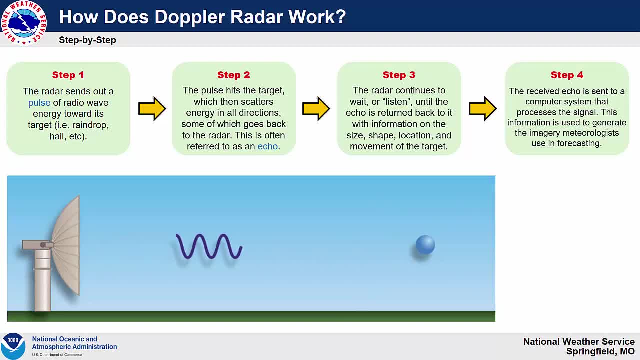 that processes the signal. This information is used to generate the imagery meteorologists use in forecasting, like the ones you see on the TV or on your smartphone app. After a few days, the radar sends data to a large radio station. This whole process is then repeated as the radar turns and makes a complete 360 degree sweep. 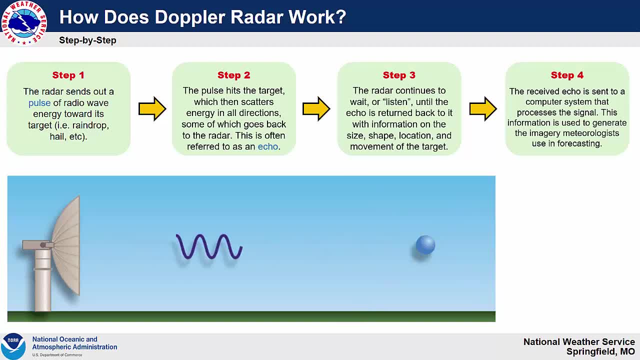 They also change the angle at which they send out pulses, allowing the radar to sample multiple elevations in the atmosphere as well. Now, I had previously mentioned in step 3 that the radar simply waits for an echo to return back to it, but did you know that radars spend a vast amount of? 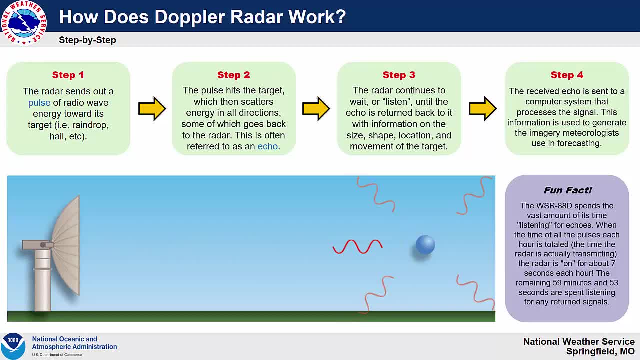 their time listening rather than transmitting. In fact, if you were to add up all the time in one hour that the radar was actually transmitting a pulse, you'd find that it only comes to about 7 seconds. The remaining 59 minutes and 53 seconds The radar is just listening for echoes. 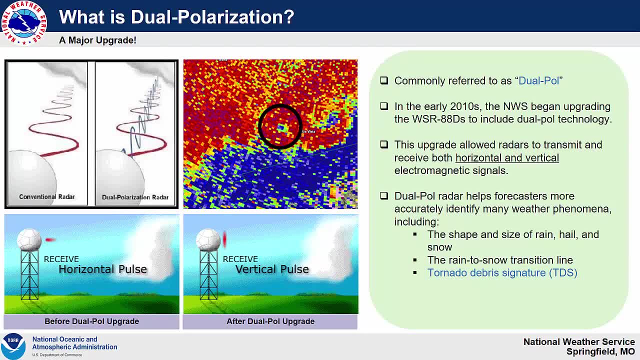 Now, if you're a fellow weather enthusiast, you may have heard the term dual polarization or dual pole thrown around from time to time. But what exactly does that mean? So when we look at the radar, it might have a pulse that is actually smoothing the pulse. 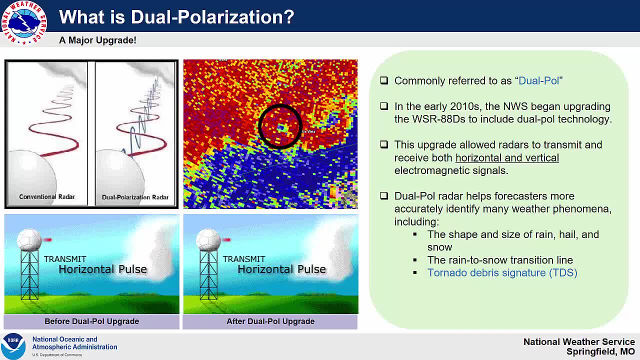 is dual polarization. Simply put, it allows the radar to measure in both the horizontal and the vertical. Prior to the upgrade, the WSR-88Ds could only transmit and receive radiation that was oriented horizontally. This limited the scope and detail we could get from single polarization radar. 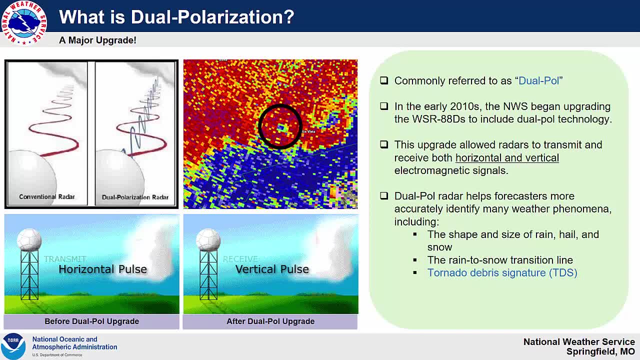 However, in the early 2010s, the National Weather Service began upgrading their radars to include dual-pole technology. This upgrade greatly expanded the information and products that Doppler radars were able to provide. For example, meteorologists were then able to accurately. 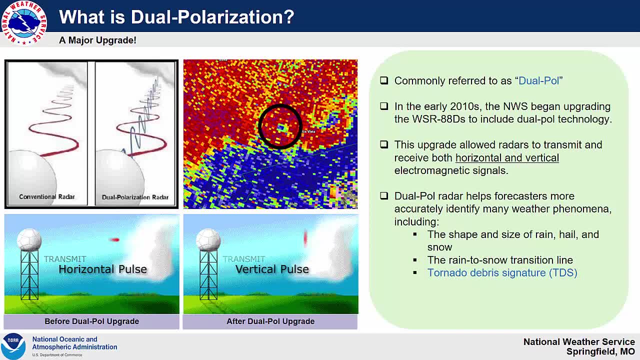 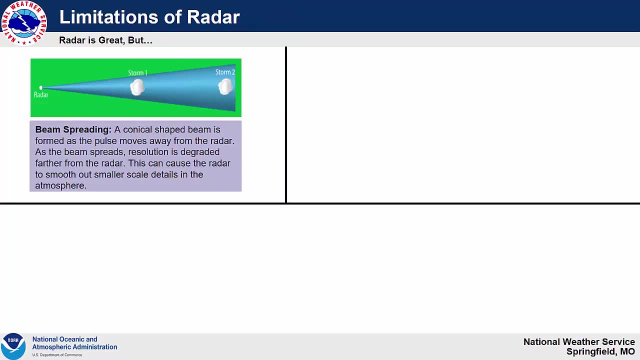 identify the shape and size of rain, hail and snow, the rain-to-snow transition line, a tornado debris signature or TDS, and much more. We'll take a deeper look at the products dual-pole provides in our next video, so stay tuned. All right, so radar is great. We as 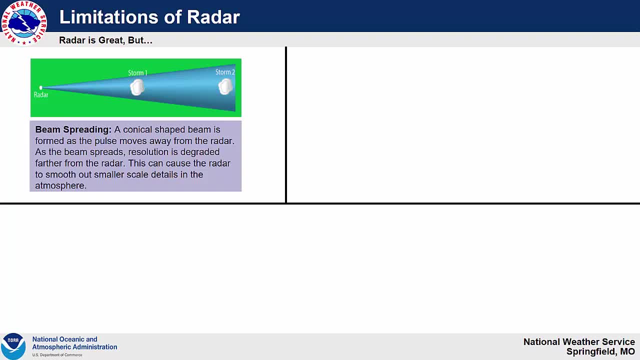 meteorologists, and meteorologists at WSR-88Ds have been able to use this technology to measure our radar. We know that meteorologists would practically be blind without it, But with every piece of technology comes a slew of quirks and challenges along with it, and radar is no. 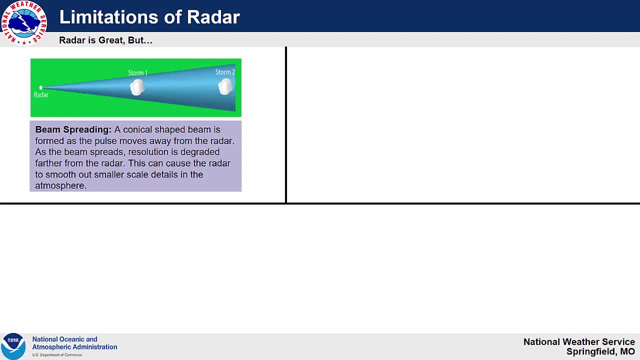 exception. Let's go over just a few of radar's limitations here. We'll start with beam spreading. A conical-shaped beam is formed as the pulse moves away from the radar. As the beam spreads, the resolution is degraded farther from the radar. This can cause the radar to smooth out. 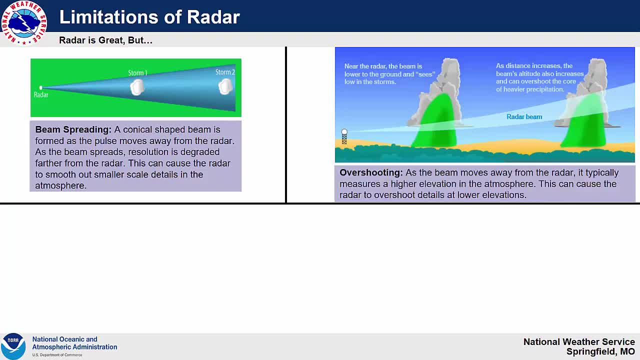 smaller-scale details in the atmosphere. Next, we have the issue of overshooting. As the beam moves away from the radar, it typically measures a higher elevation in the atmosphere. This can cause the radar to overshoot details at lower elevations, which can especially be a problem when looking at severe thunderstorms. 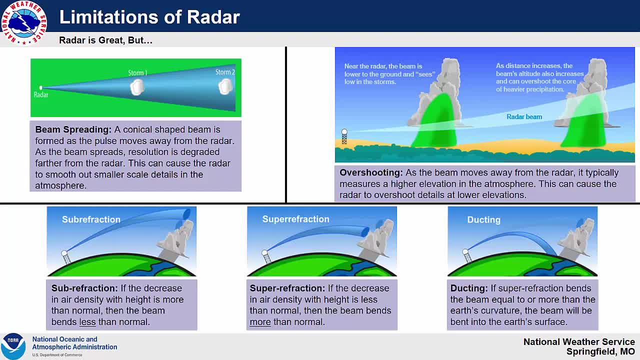 Finally, there's refraction. Refraction is simply when light or radiation is bent as it passes through mediums with different densities. Therefore, since the density of the atmosphere is atmosphere is not the same everywhere, this can cause the radar beam to be bent in several ways. 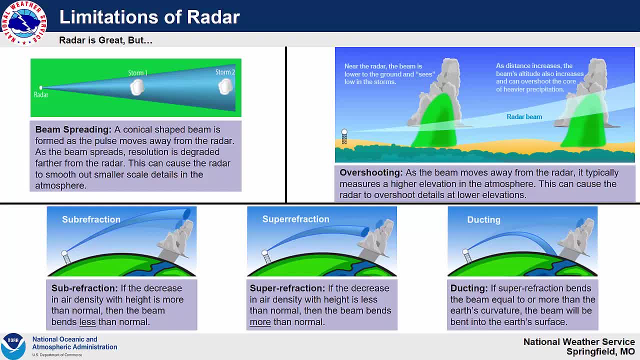 Subrefraction is when the decrease in air density with height is more than normal, causing the radar beam to bend less than normal. Superrefraction, on the other hand, is when the decrease in air density with height is less than normal, then the beam bends more than normal. An extreme case of 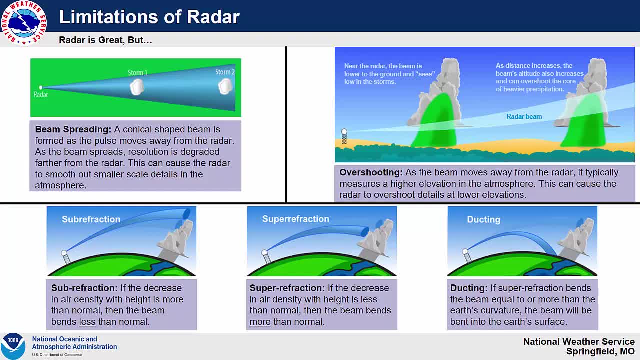 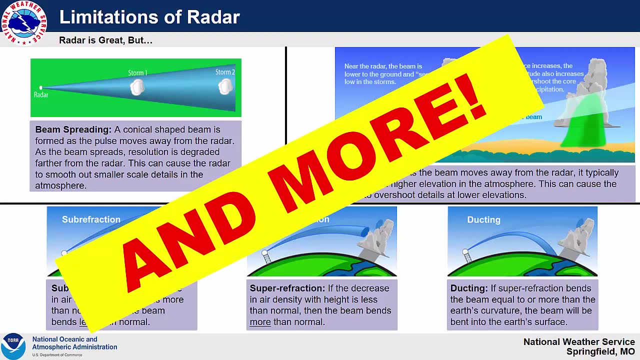 superrefraction is called ducting. Ducting is when the beam bends more than the earth's curvature. As a result, the beam will eventually be bent into the ground. This can cause some very unusual signals to be turned to the radar. There are many more things to keep in mind when looking at radar.